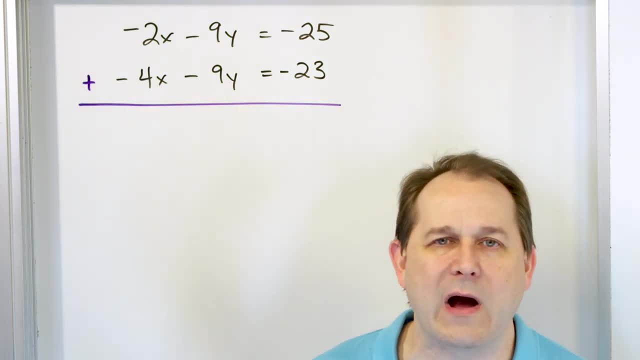 And so you will have a new equation that will still have x's. You'll have a new equation that will still have y's, and you can't do anything with it. What do we do? Okay, what you have to do is change one of the equations in order to make it cancel one of these terms. 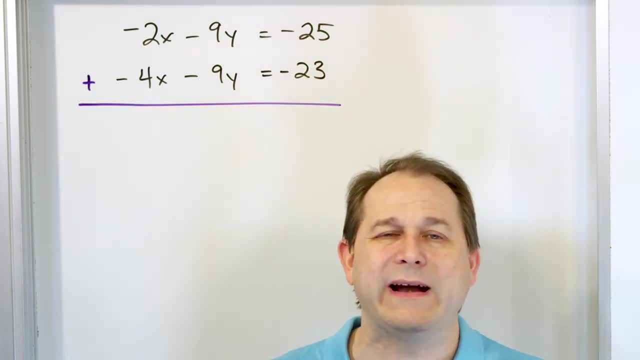 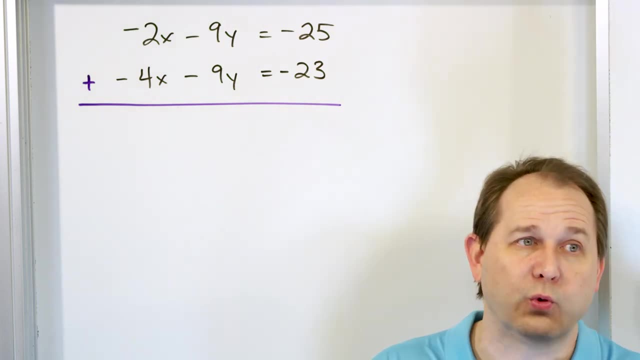 And that's why I say there's like a little step you have to do in the beginning here. If it doesn't already set up, if it's not already provided to you so that something will cancel, then you have to do something that is legal within the rules of algebra to change one of them. 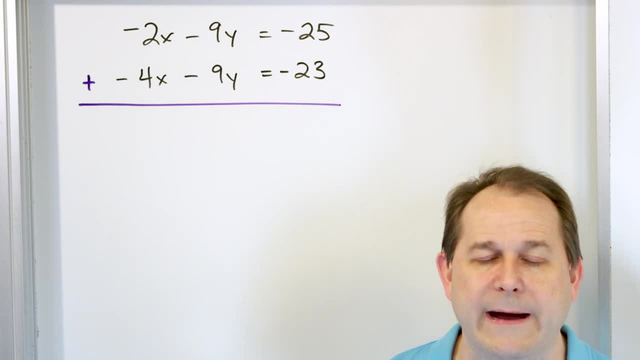 so that when you add them together, one of those terms will drop away. Now you can add things to both sides of an equation. You could subtract, You can also multiply on both sides of an equation by anything you want, and you can also divide both sides of an equation by anything you want. 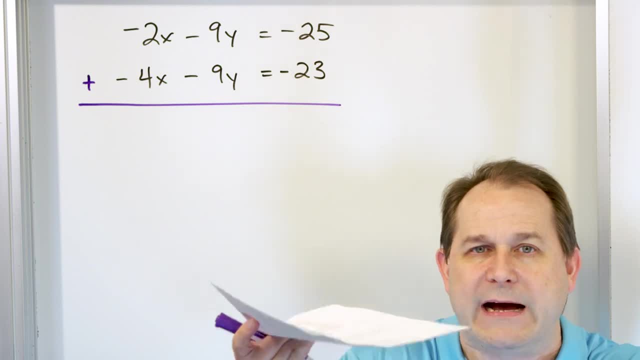 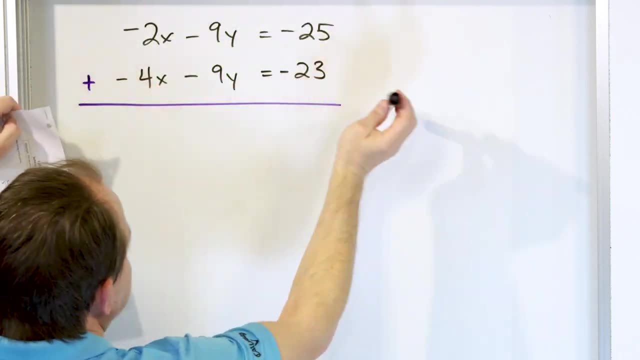 That's legal. We know that multiplying or dividing both sides keep the equation balanced. So what would happen if we just took this equation- this top one or the bottom one doesn't matter, but the top one? what would happen if we actually multiplied this equation by negative 1?? 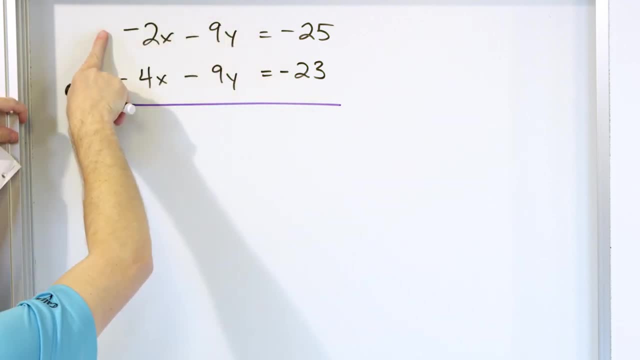 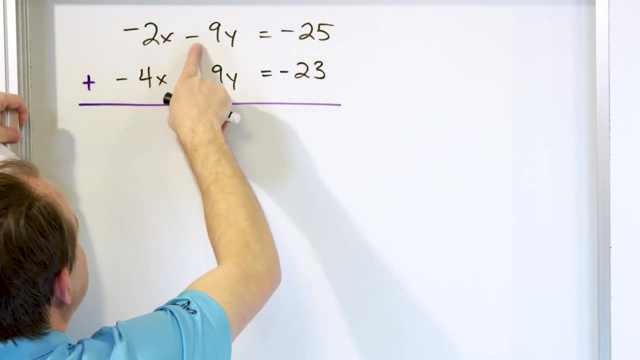 Well, if we multiply by negative 1,, it means we multiply the left side by negative 1, and, to keep it balanced, We also multiply the right side by negative 1.. What will happen is we're going to flip the sign of this guy and then it'll be positive 9y. 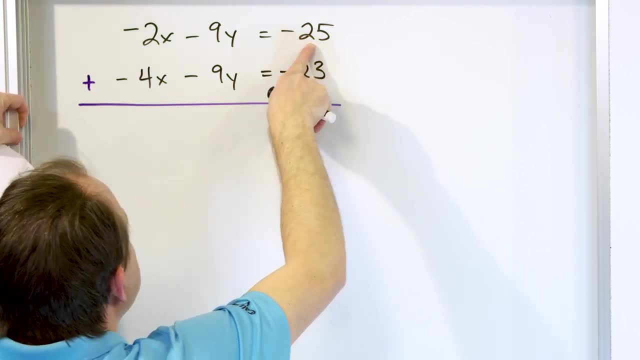 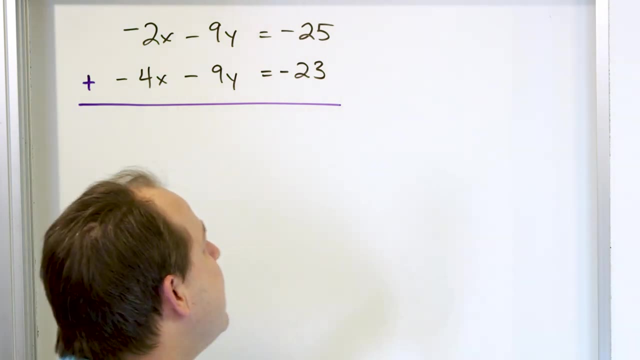 here and positive 2x, and this will be positive 25, and it looks different. but we can multiply by negative 1 on both sides, because we know we can multiply both sides by anything we want. But by doing that we get a positive 9y which we can then add to here and kill it and make it go to 0. 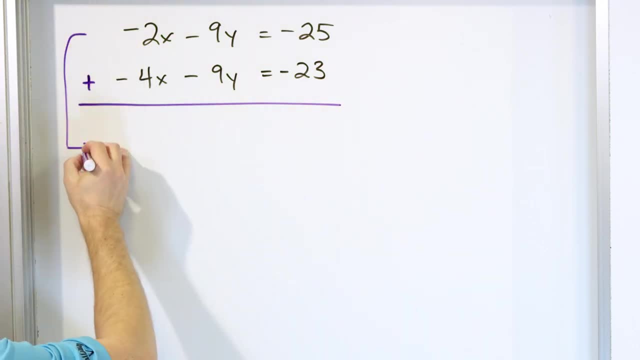 So the actual first step is not to add these things at all. It's to take the left side and multiply by negative 1.. And what you're going to do is multiply it times the left-hand stuff. But if you're going to multiply the left by negative 1, you have to multiply the right by negative 1.. 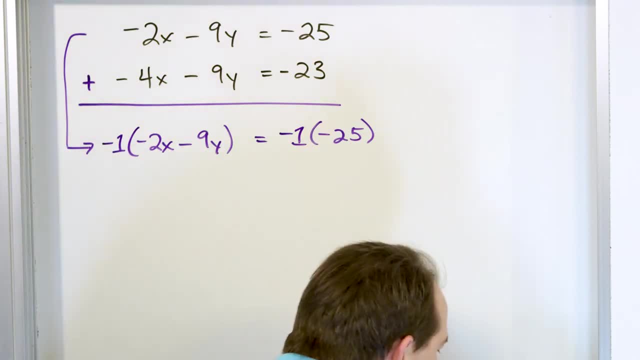 Otherwise what you have is not legal. All right. so what happens when we multiply by negative 1?? Don't forget, you have to distribute, It has to be everything multiplied by negative 1.. So this becomes a positive 2x, and this times this negative becomes a positive 9y. 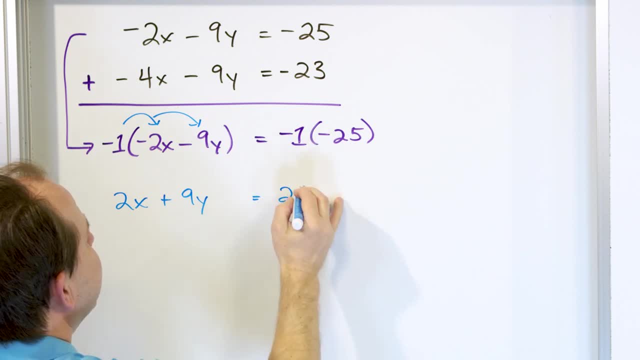 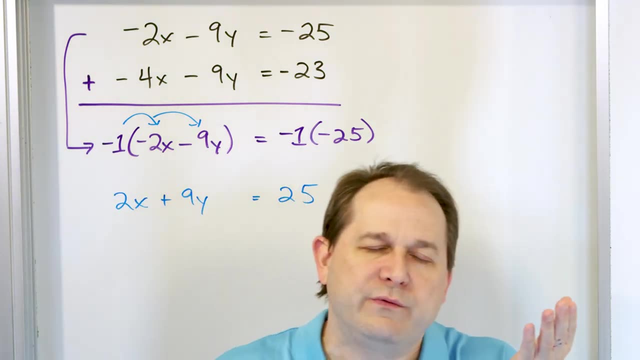 and this on the right side of this: x will be positive 9y and the equal sign becomes a positive 25.. Now this equation looks different than this one, but actually it represents the same thing, Because when you take both sides- yes, you did change all of the signs on the left-hand side. 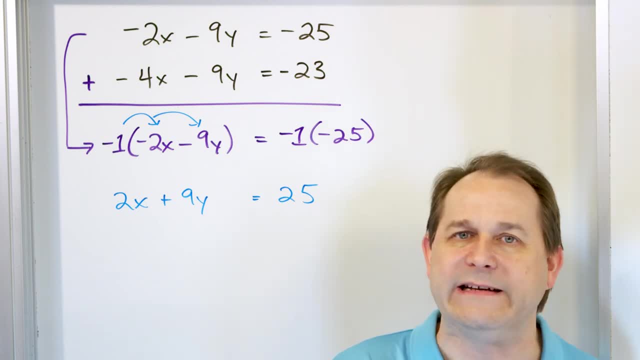 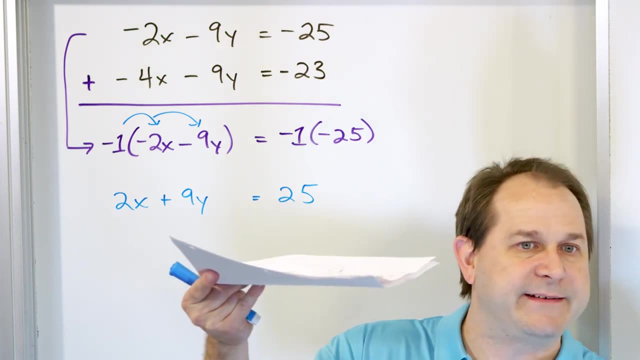 you made them all negative, but you also, at the same time, made the right side negative too. So the equality that you had there is preserved, because it's just like a scale: If you multiply by something on one side, as long as you do it to the other side. 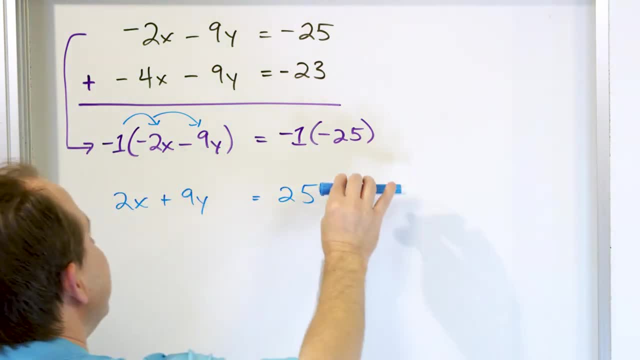 then it looks different, but it actually represents the same thing. These two things are the same thing, really, even though they look different. So then I'll just write this other equation down below, and I won't change it because I don't need to. 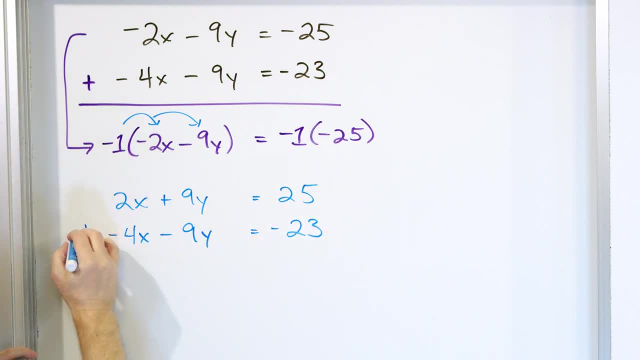 I have a nice cancellation here And now I can add these blue equations together. So I basically changed the top equation into something new and now that when I add these together, of course it all works out now. So two x plus this. 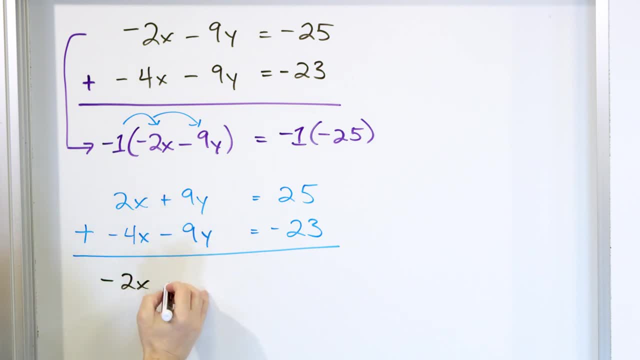 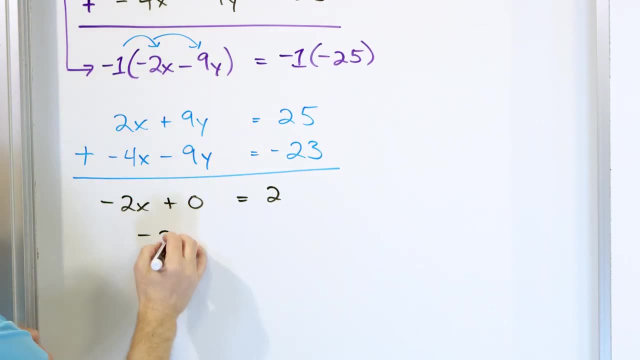 negative four x is gonna give you negative two x. When we add this together, we'll get a zero Zero y. And then over here, when you add this, you'll get a positive two. So you have negative two. x is equal to two. 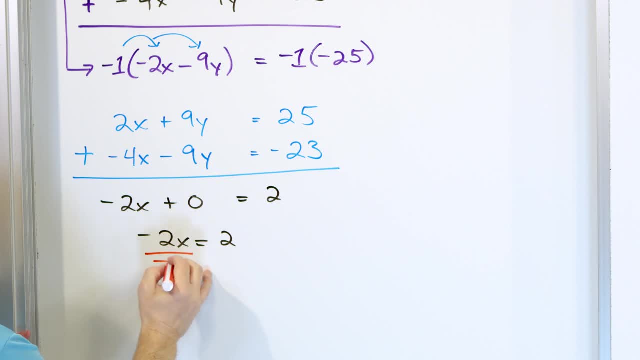 How do I solve this equation? Well, I'll just divide by negative two And what I will get is cancellation on the twos You'll get, x is equal to negative one, like this negative one. Now the rest of the solution proceeds as usual. 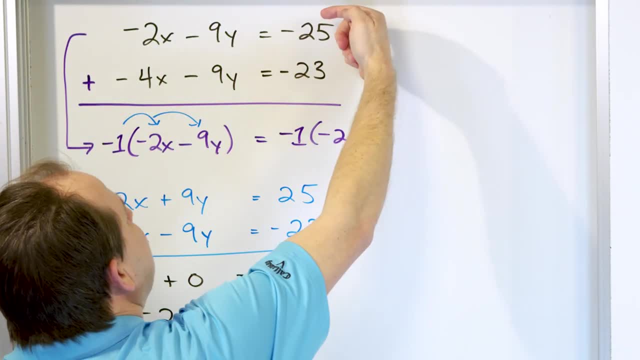 I can take this. x is equal to negative one. I can put it into anything I want. I can put it into here. I can put it into here, or I can put it into here. I can put it into here. I can put it into this version. 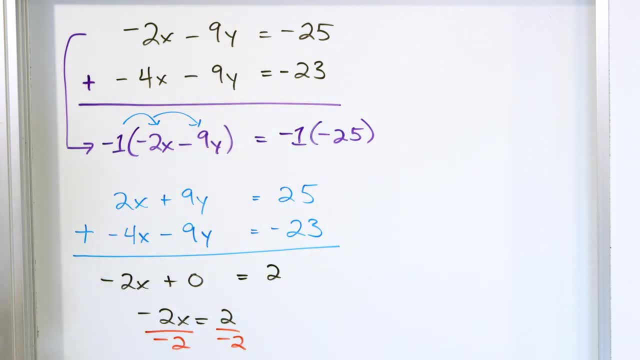 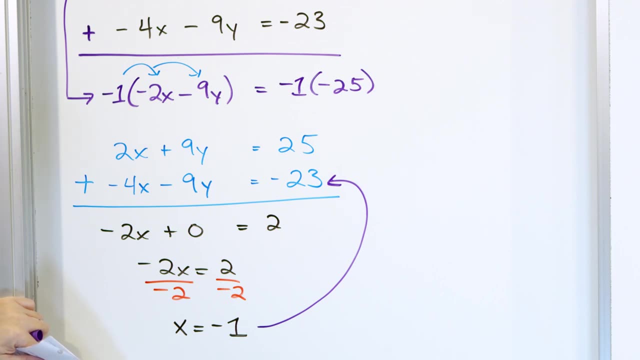 which is slightly different, or this one. I'm gonna get all the same exact thing, no matter what I do. So I'm gonna take and stick it into this bottom one, just because it's the closest one. There's no real reason, no real preference. 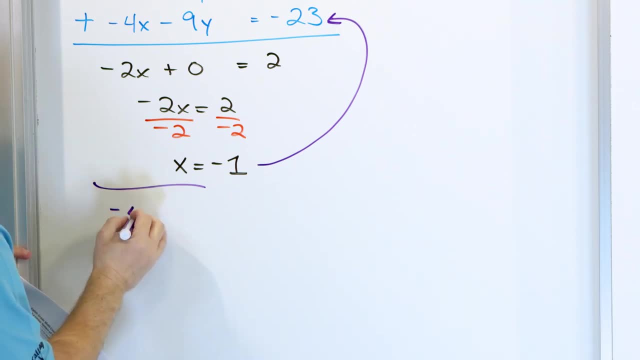 It's all gonna be the same. So what we will have is negative four times x, but I know that x is now negative one minus nine times y here, and then it's equal to negative 23. This becomes positive four minus nine y. 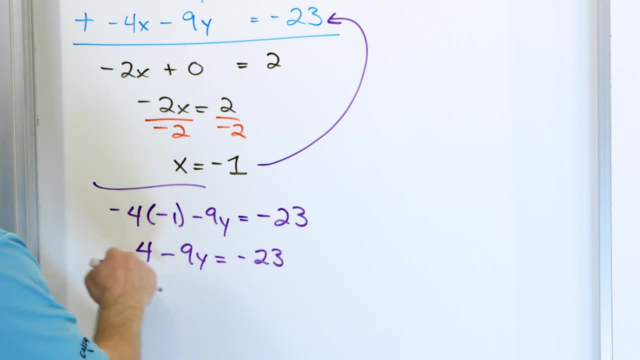 negative 23.. All right, How do I get rid of? how do I solve this equation here? Well, what I'm gonna do is I'll just- since this is plus four, I will actually I think I'm gonna- rewrite this guy. 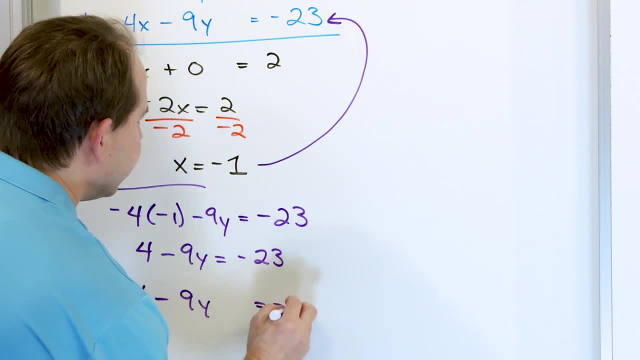 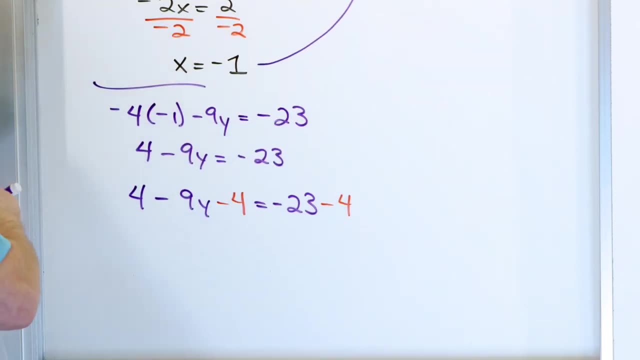 It would be four minus nine y, negative 23.. So what I'll do? since this is positive four, I'll get rid of it by subtracting four, subtracting four. So the negative nine y will be what is left. Four minus four is zero. 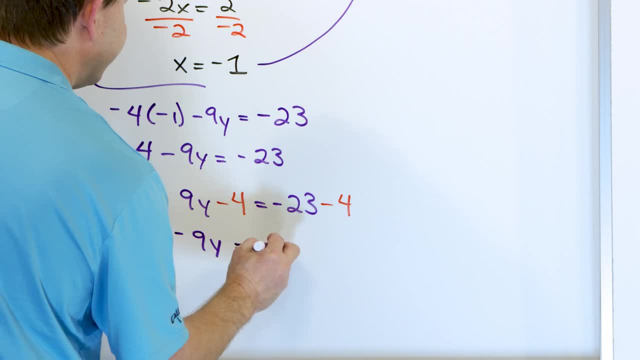 And then negative 23 minus four is negative 23.. I'll get rid of it by subtracting seven And I'll just read and write it in like the way it should, And that is going to end up being negative two times three. 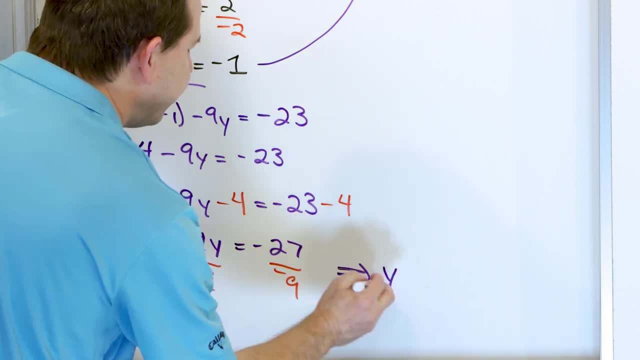 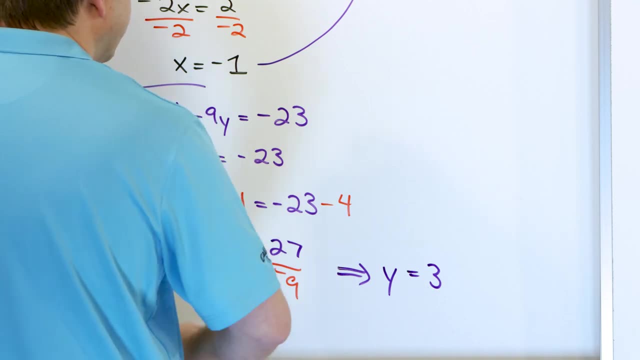 minus six times x, plus four times x, minus five times x, And then I'll just keep writing it over. I've got zero, and then I can turn this in to my equation. I have negative nine times x because I stopped having anything negative before. 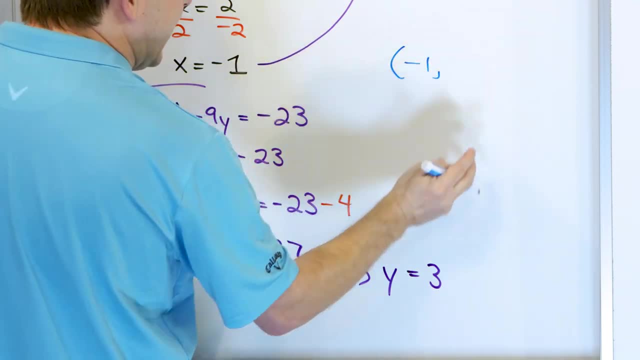 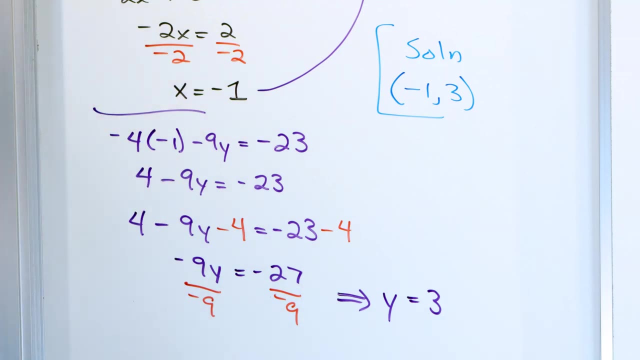 All right, I'm gonna write back the answer to divide the 57, and I'll just start on this and then divide it over. I get 12 and 3 times four times x negative 1 comma 3. so this procedure: it follows exactly what we did before. we're still adding the. 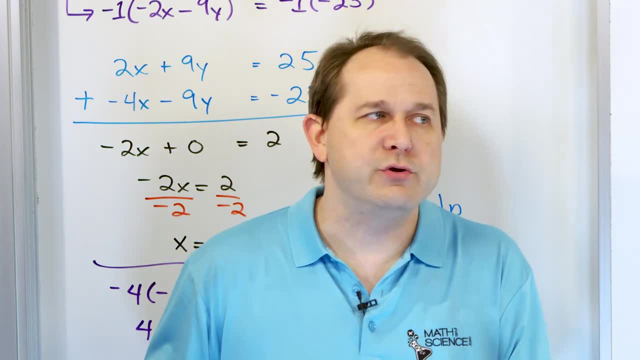 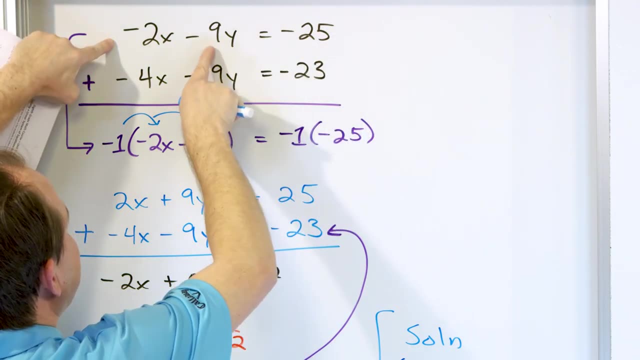 equations, everything is the same. the only thing is, because you know that you can multiply an equation by anything you want, we're going to choose. as long as you do it to both sides, we're going to choose because we have a 9 here. in both cases, we're going to choose to multiply this by. 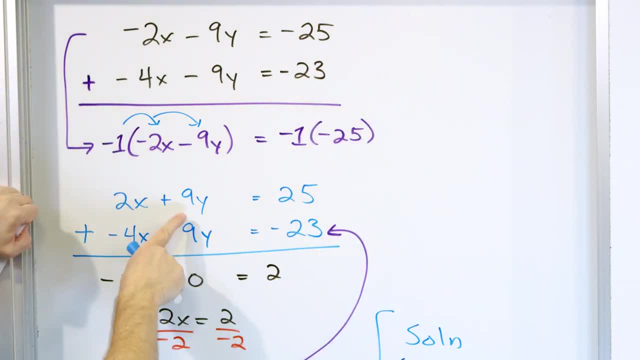 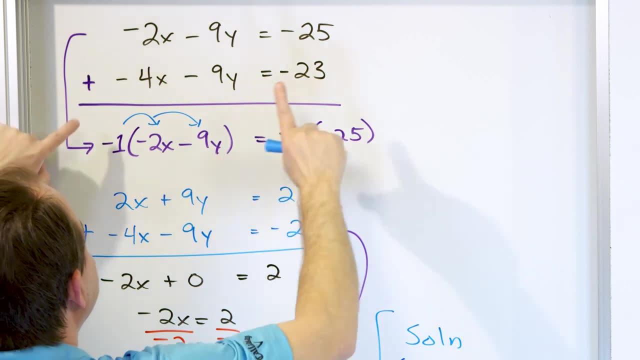 negative 1, because by doing that i flip the sign of this, so that when i add it i will get the same thing. now let me go back and say i don't have to multiply this by negative 1. if i wanted to, i can instead choose to multiply this one by negative 1. that will flip the sign of this. 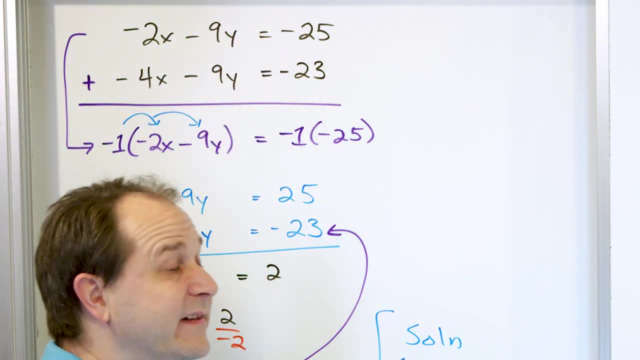 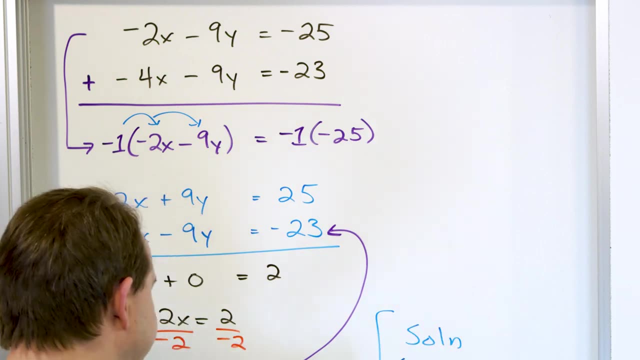 and i'll add them together and if you go through it, you're going to get exactly the same answer. as long as you're doing legal things, you will always get to the same answer, so don't stress out about which one to work with: both will yield the correct answer. all right, let's take a look. 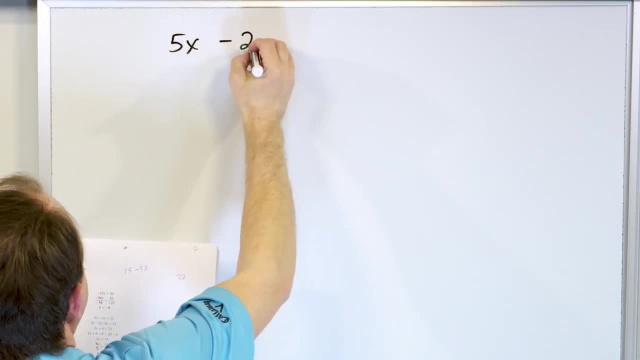 at the next problem: 5 times x minus 2 times y is equal to 23, followed by 5 times x plus 8 times y minus 2 times y is equal to 23 plus 8 times y minus 2 times y is equal to 23. 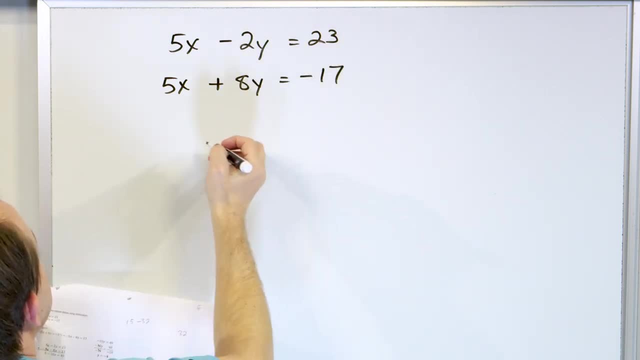 plus 8 times y minus 2 times y is equal to 23, followed by 5 times x plus 8 times y. plus 8 times y is equal to negative 17,. all right, So what am I gonna do right here? If I add these straight away, five plus five is 10x. 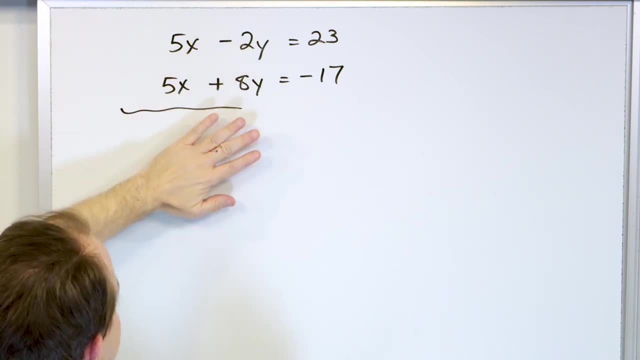 and then this will give me six y and nothing's gonna cancel the variables won't cancel. So I have choices here. but the easiest thing to do is to recognize I have two fives here, two five x's, So I can either multiply the top equation by negative one. 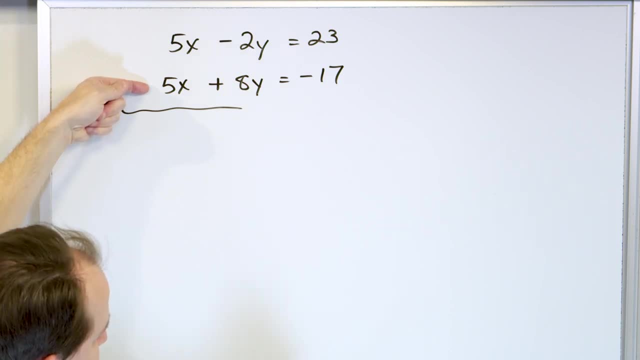 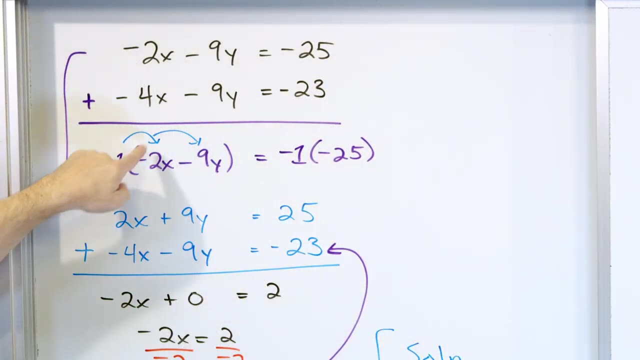 or I can choose to multiply the bottom equation by negative one, and both of these guys will give me exactly the same answer. Now, in the previous example, I took the first equation and multiplied it by negative one to flip this guy. I could do that here, but just to make it different. 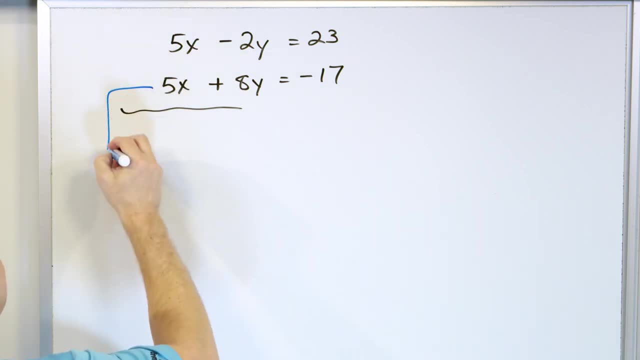 let me work with the second equation right here. Let me just take that second equation and show you. it doesn't matter which one you do. I'm gonna multiply negative one. five x eight times y, and then you have to multiply the other side as well. 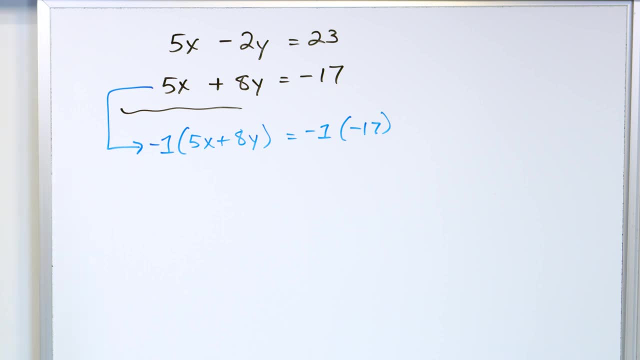 because you can multiply both sides as long as you do it to the same thing, to both sides. So what do I have? Negative one times- the five x is negative five x. and then I have negative one times. this is negative eight times y. 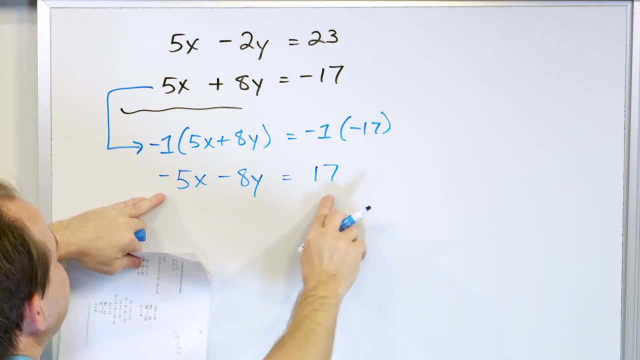 and then I have over here positive 17.. So this is the new equation, which is different looking than this one, but actually represents the same thing. So what I'm gonna do is, since I have this equation written from here, I'm gonna grab this equation. 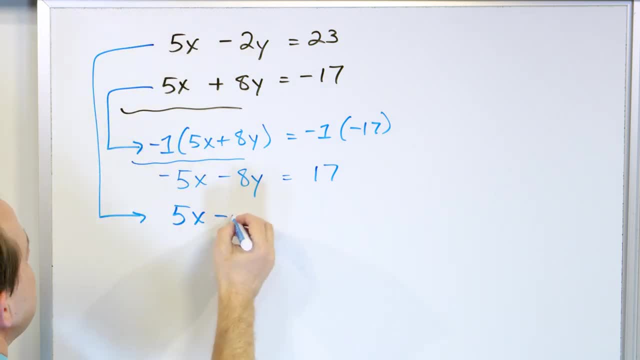 from the top and bring it down and just write it underneath: five x minus two y is 23, and I'm gonna add these equations together. So what I did is I took the bottom equation, I multiplied by negative one. here's what I got. 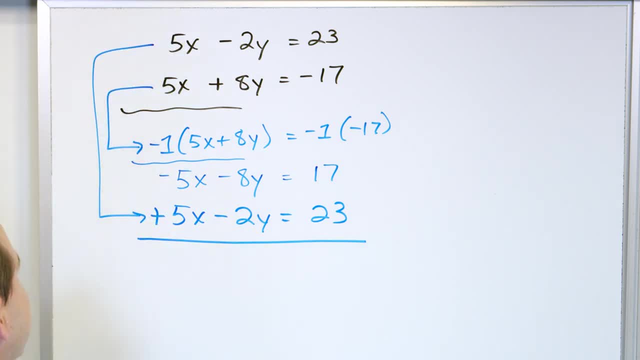 and then, once that was the second equation, then I take the top one and write it down underneath and I add: negative five x plus five x is zero. negative eight y plus a negative two y is negative 10 times y, and then 17 and 23 is gonna be 40. 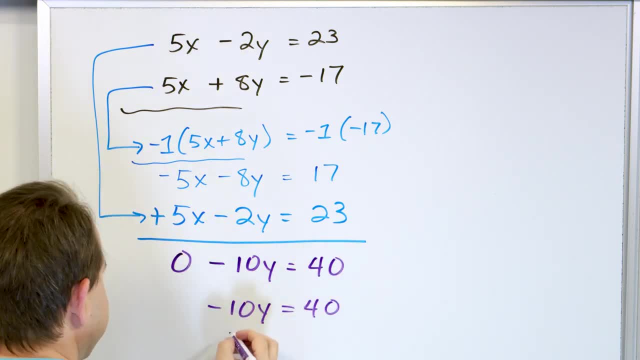 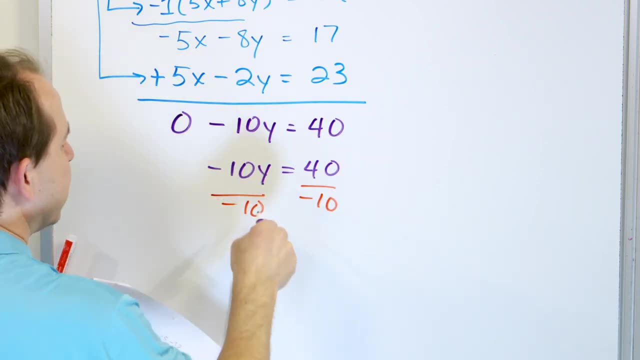 And so I have negative 10 times. y is 40. How do I solve this equation? I'm gonna divide by negative 10.. The 10s will cancel, the negatives will cancel. I'll have: y is equal to. this is negative four. 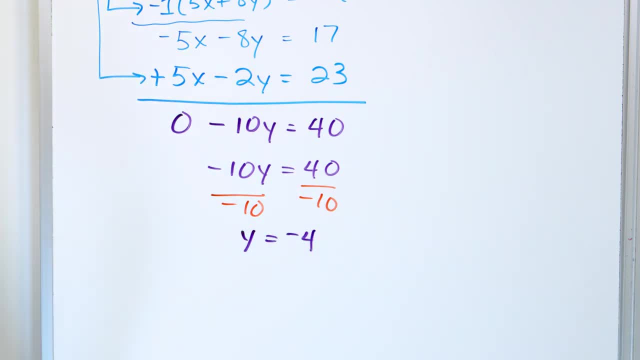 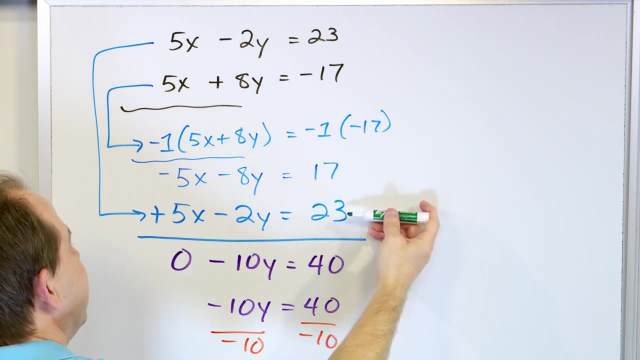 Y is equal to. let me just double check myself: negative four, That's correct. Then I can take this negative four and I can put it anywhere I want. really, I can put it into either one of these equations or I can put it into either one of these. 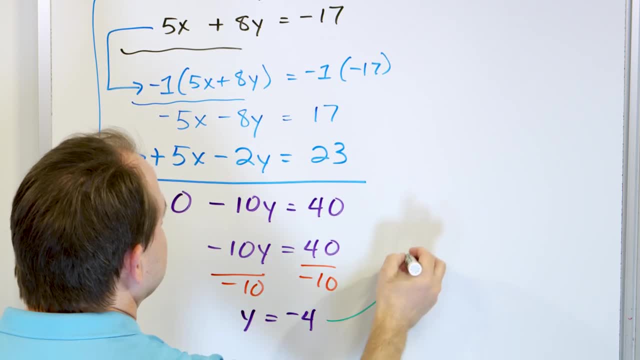 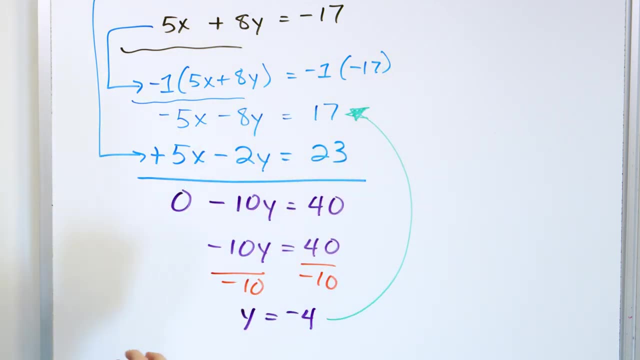 I will get the same answer. So let's just put it into this one. just to do something different. We'll put it into the top equation right there, but I could put it into this one, That'd be fine. So I have negative five times x minus eight here. 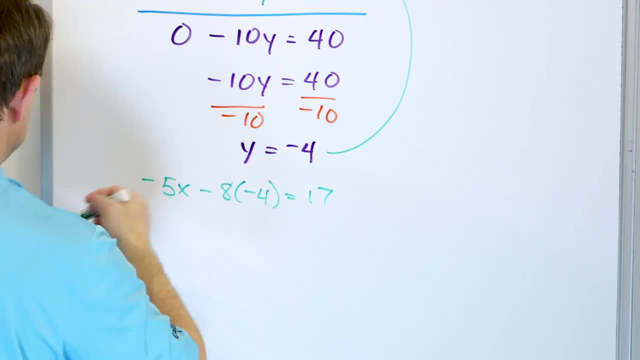 times y, which is negative, four is equal to 17.. So negative five times x, this becomes positive. 32, is equal to 17.. So I'm gonna have: negative five times x plus 32 is equal to 17.. Now to get the number over here. 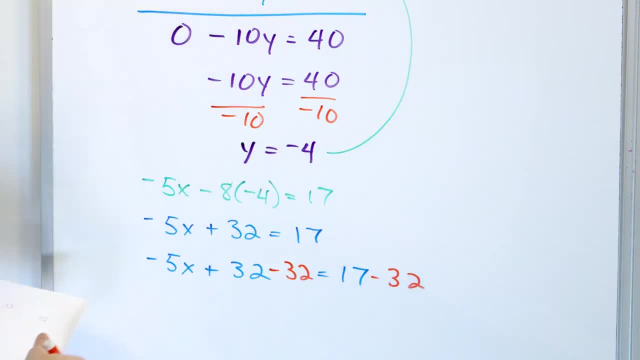 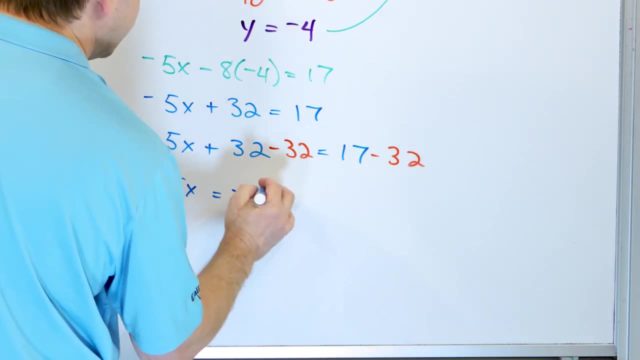 I'm gonna subtract 32,, subtract 32.. So this goes to zero. Here I'm gonna have negative five times x, and on the right-hand side, right here, I'll have negative 15.. Now how do I solve for x? 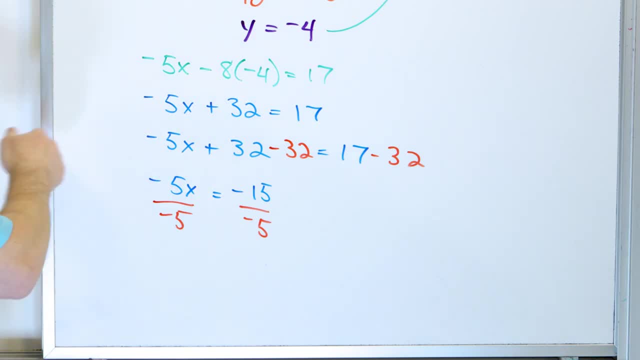 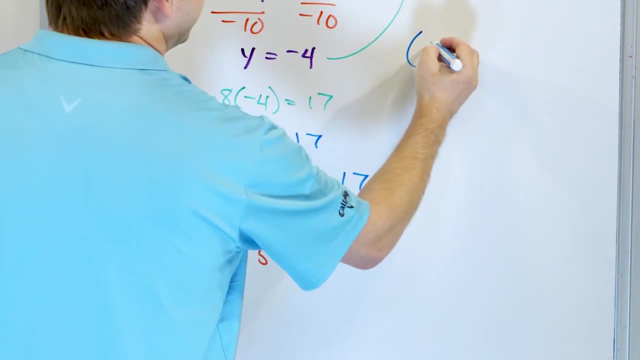 I'll divide by negative five And when the fives cancel here, I will have a value of x. of what is this? Positive three, positive three. So, putting it all together, an x value of positive three and a y value. 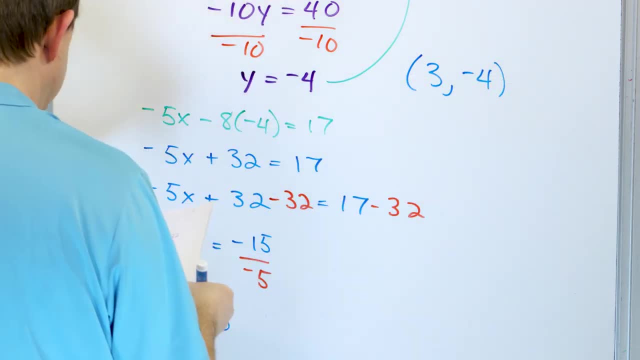 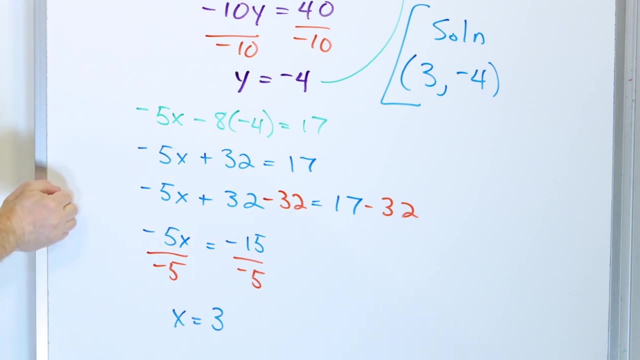 which I already solved for, of negative four. this is my point. three comma, negative four. This is the solution. This is the intersection point of both of these lines. Okay, let's take a look at problem number three. So so far we've had two problems. 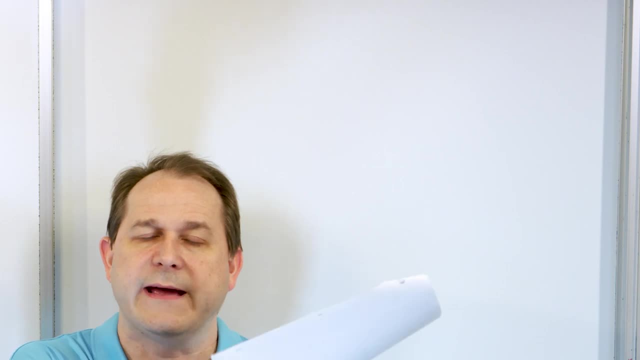 both of which have intersected, and we have two lines that are intersecting in one point. We're gonna do one more of a similar form And the last problem that we have- I'm gonna give you a punchline ahead of time: It'll be parallel lines. 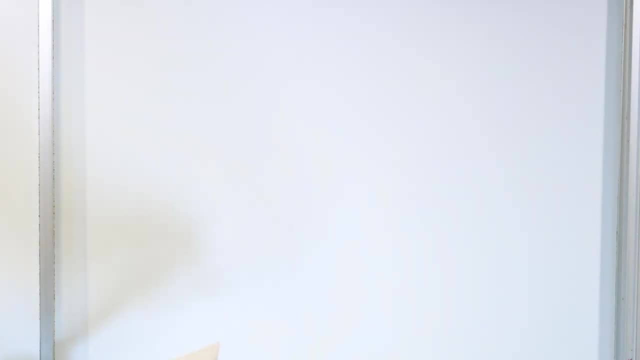 And we're gonna see what happens when there's no solution at all. All right, problem number three. let's take a look. It's three x minus seven y equals negative two, and six x plus two y- negative 20.. Now if we just add these straight away, 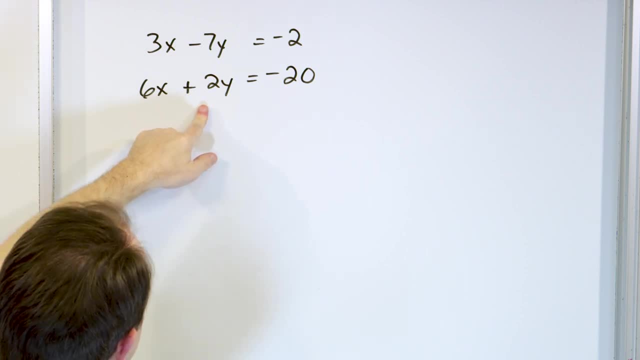 we're gonna get nine x And then this plus this will be negative five y, And then we'll add these, but nothing will cancel. No variables will cancel. But this is a little different. We can't just multiply one of these by negative one. 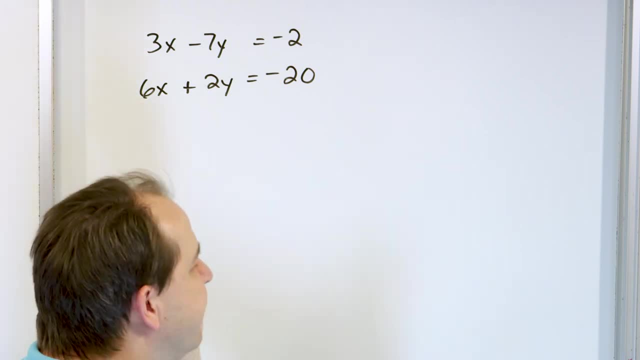 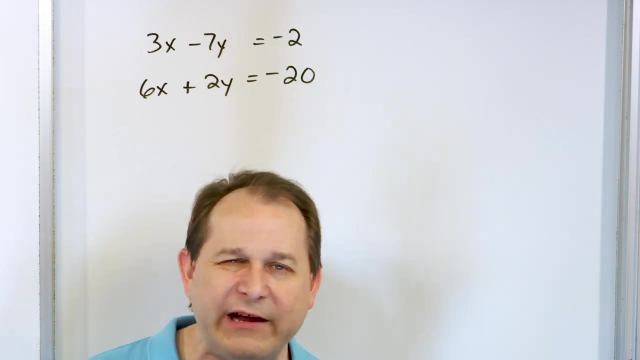 because if we do that, we still won't get any cancellations. So is there any other number? we can multiply, We can manipulate these equations, just like fractions. right to change them. We'll change one of these guys. What do you want to do? 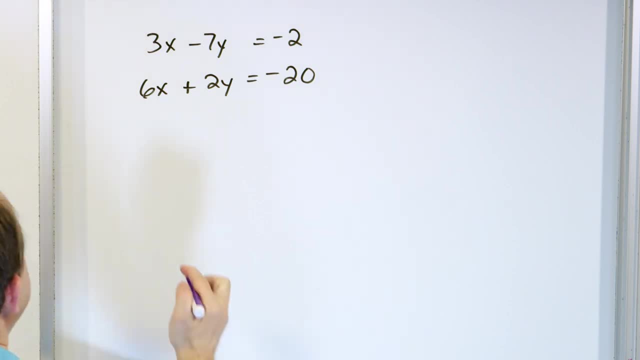 Let's, instead of just trying to multiply by a negative one, let's take this top equation and figure out what we can multiply it by. Let's write down: three x minus seven: y is equal to negative two. What can I multiply this equation by? 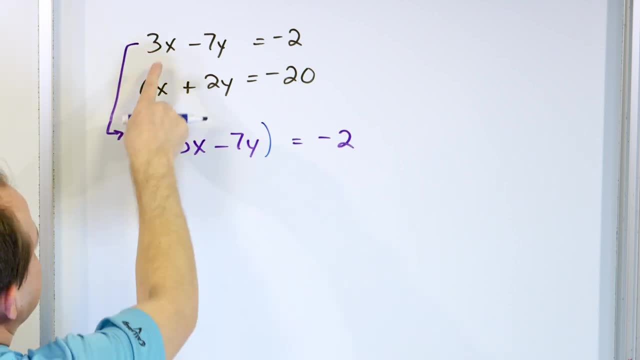 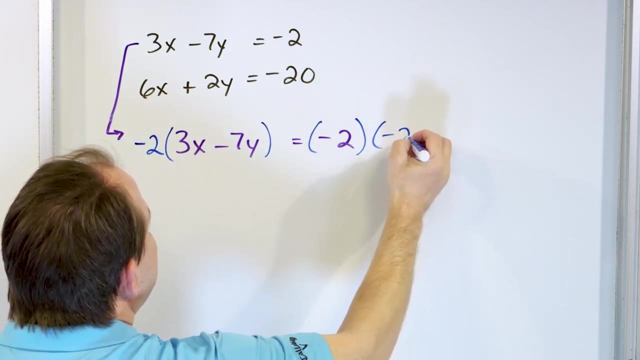 so that when I add it to the six it's going to kill the term. here I have to multiply by negative two, And if I do it to the left I have to multiply by negative two on the right. So when I multiply this out, 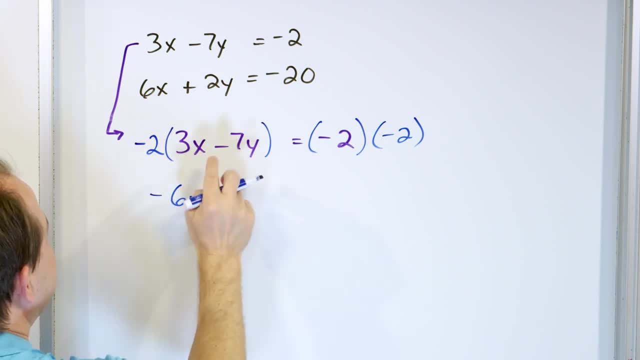 I'm going to get negative six times x, And then this times this is positive two times seven, 14 y, And then this right here is positive four. So this equation, even though it looks totally different, really is the same thing as this one. 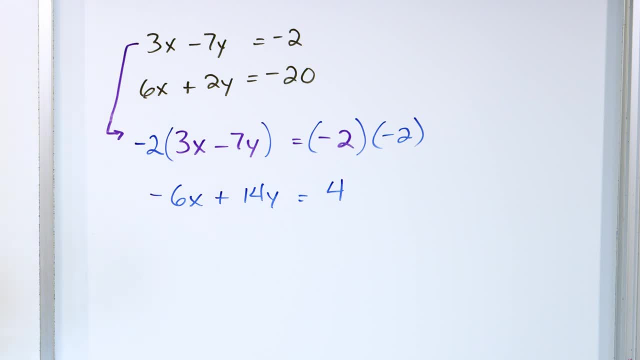 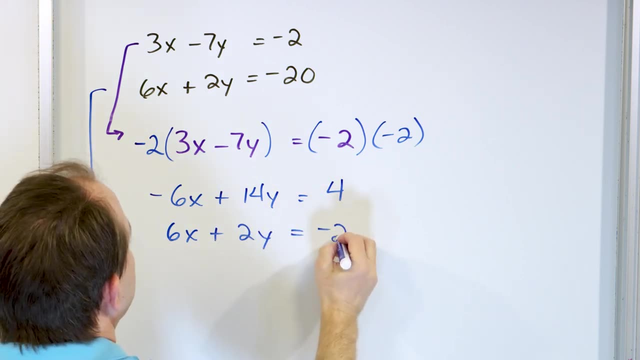 because we multiplied by a common number to both sides. Now let me take this equation and write it down underneath: It's positive six x plus two y is negative 20. And then you can see that you can add these guys together, because now they will cancel. 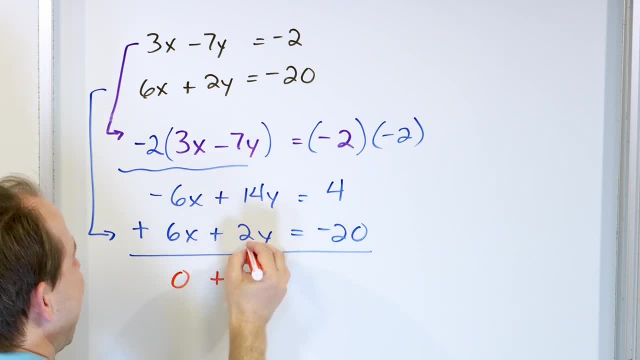 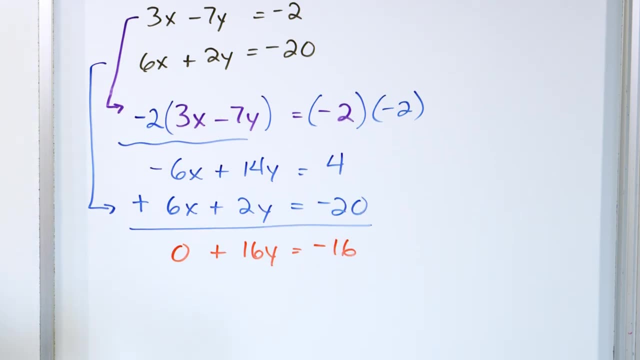 So when I add them together, I get zero here, And then when I add these, I get 16 times y, And when I add these four plus a negative 20, I get negative 16.. So I will have: 16 times y is negative 16.. 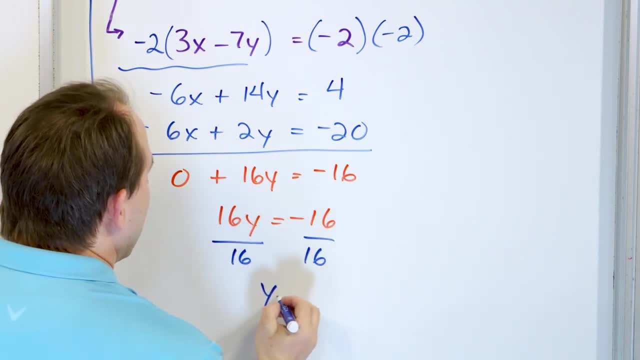 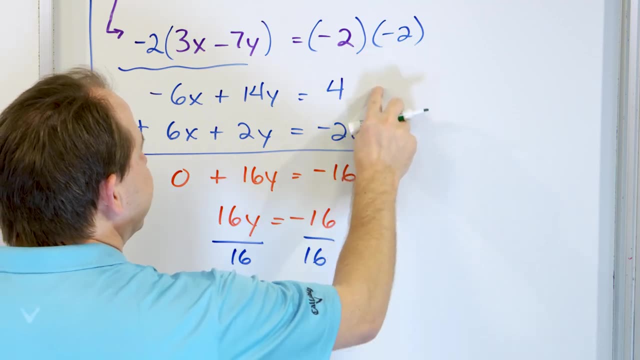 And then when I divide by 16 to get rid of it, y is negative one. The answer is negative one. The answer is negative one for y. Now I can take this thing and I can put it into either one of these equations or either one of the original equations. 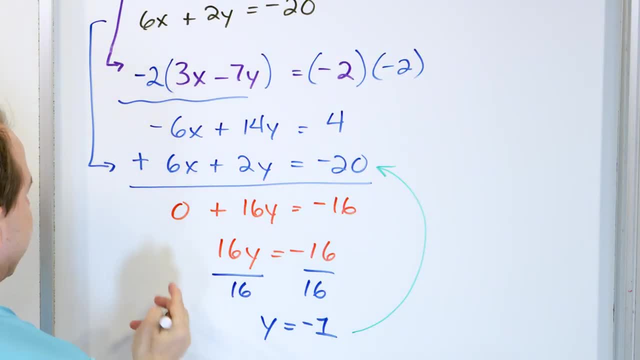 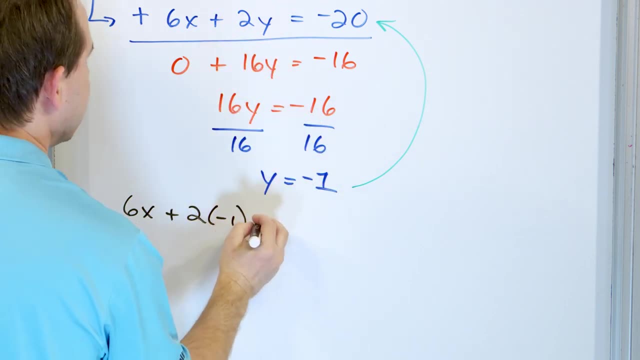 It's going to give you the exact same thing. Let's put it in here and see what we get. So here we have six times x plus two times y, but we know that y is negative, one is equal to negative 20.. Six x minus two from here is negative 20.. 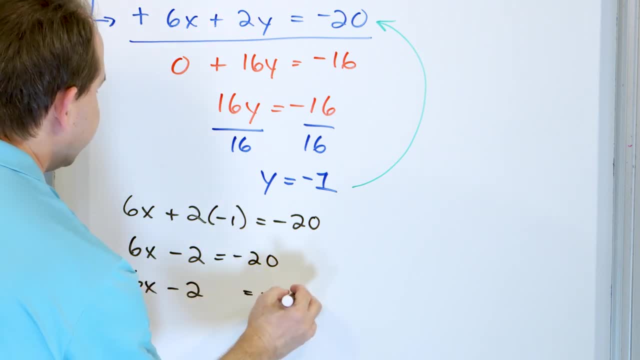 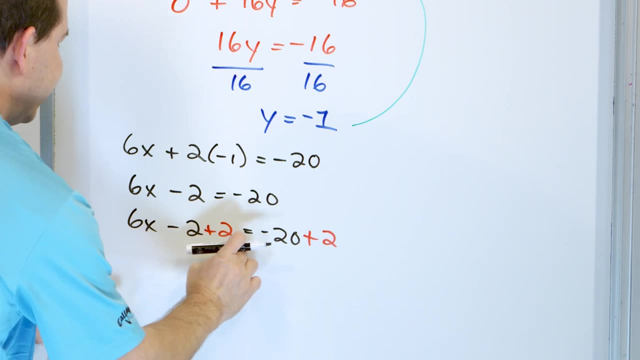 Now we have six x minus two, Minus two negative 20.. We want to solve this equation, So we're going to add two, add two, And of course we get zero here. So we just get six x. And on the right-hand side, what do we get? 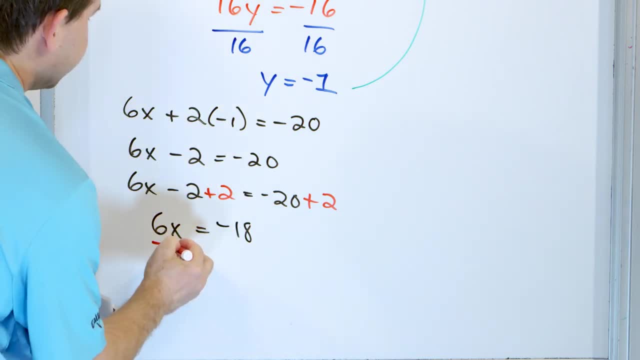 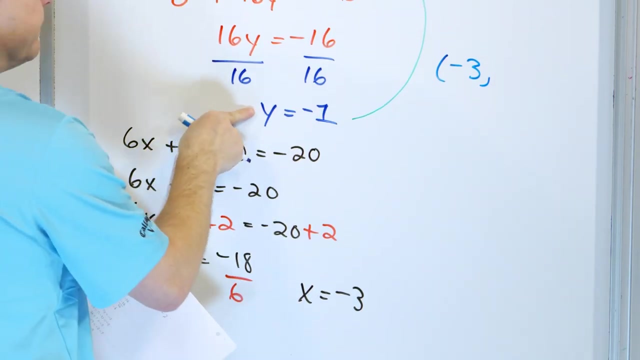 Negative 18.. So how do we solve this one? We divide by six, divide by six And when we cancel here we get a value of x is negative three, Negative three. So when we put it together we say the x value of negative three and the y value 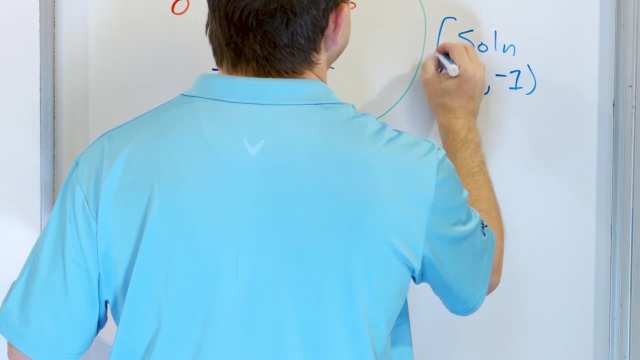 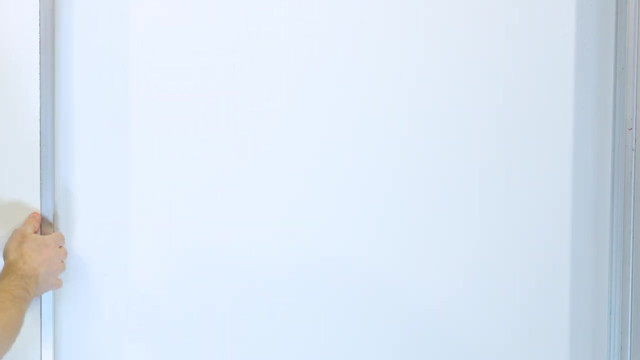 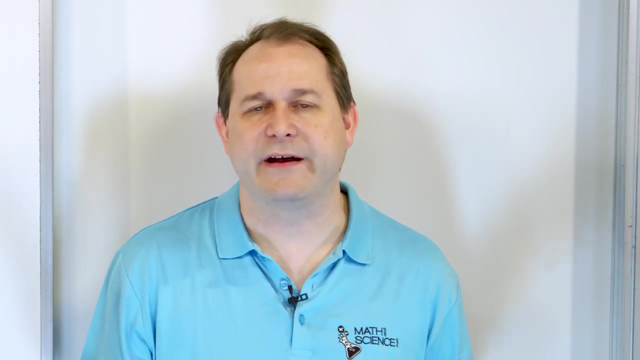 is negative one. This is the solution: Negative three comma, negative one. So up till now all of these problems have had a single intersection point And we learned before that if two lines are parallel and they never cross, they don't have an intersection point. 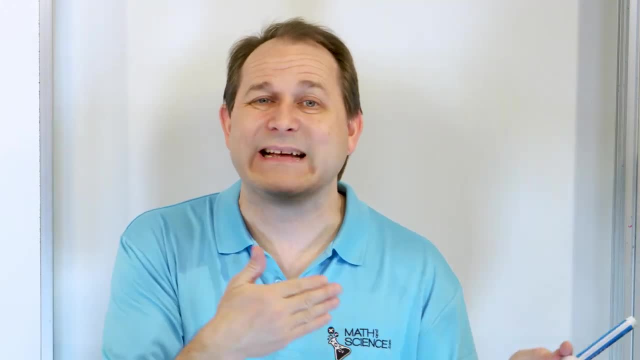 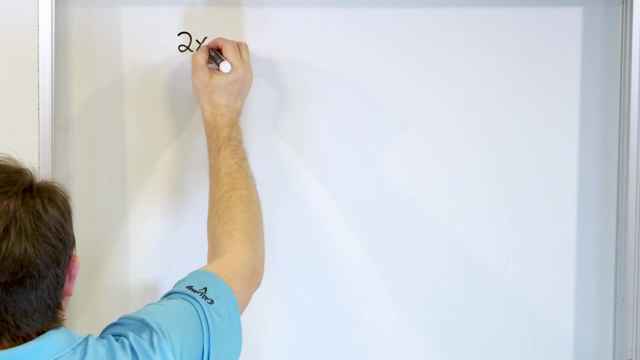 And so there's no solution. It's really easy to see when you graph it, but let's see what happens when we try to solve a system like that. Right here's our last problem. Two times x plus- Okay, 3 times y equals 8.. 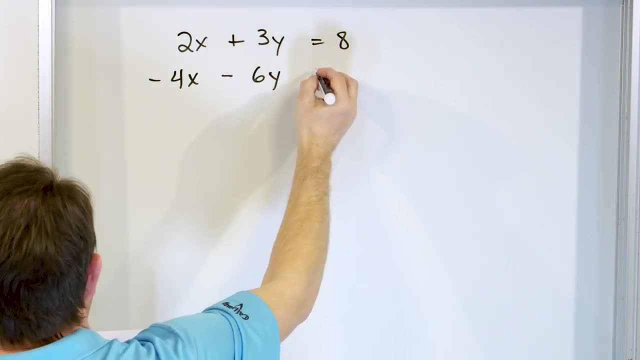 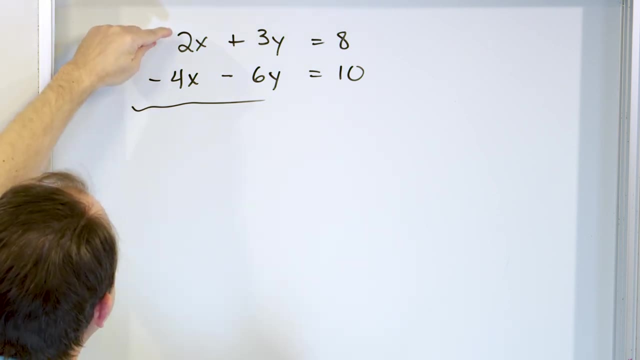 Then we have negative 4 times x minus 6 times y equals 10.. So we have no idea what this thing looks like, But we know that we have some choices. See, if I multiply this by 2, then I'll have 4x. 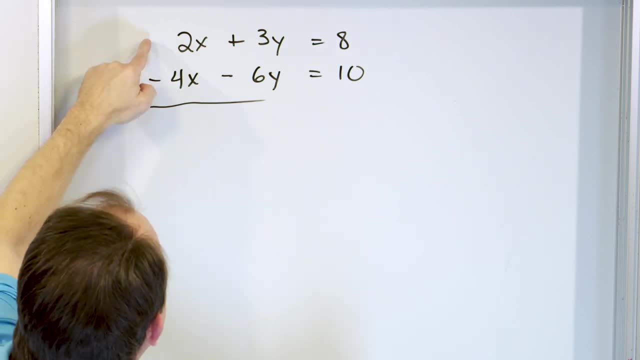 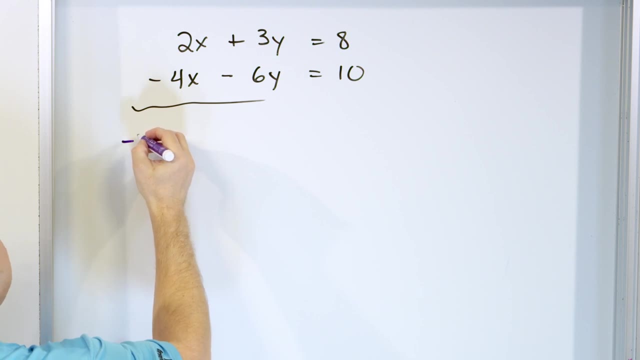 And I will be able to cancel with this when I add it If I multiply this by 2, we know that that's going to happen, So let's go ahead and do that. So if I take and multiply positive 2 times 2x plus 3y. 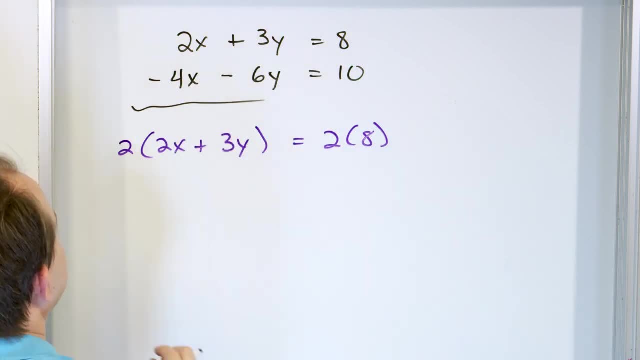 And then if I do it to the left, I have to do it to the right. I just multiplied both sides by 2.. So what I get when I do that? multiplying here, I get 4x. Multiplying here, I get 6x. 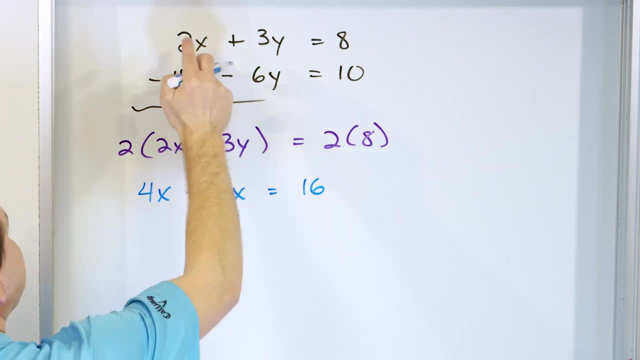 And then over here I get 16.. So I've multiplied the first equation. Let's now take that second equation and put it in here: negative 4 times x, Minus sign: 6 times. whoops, sorry, I made a mistake. 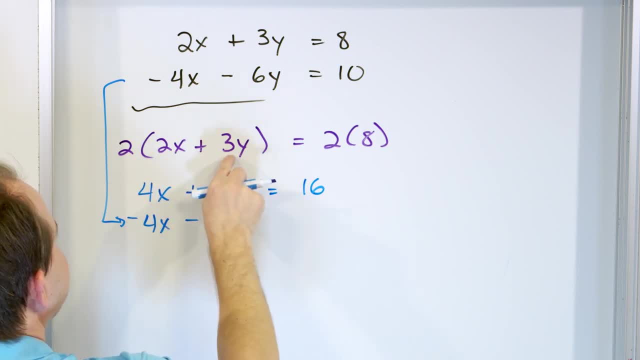 This should be not an x, Because 2 times 3 is 6.. This should be a y, And then this one is negative 6y, And then this 10 comes down here. So let's add both of these equations together. 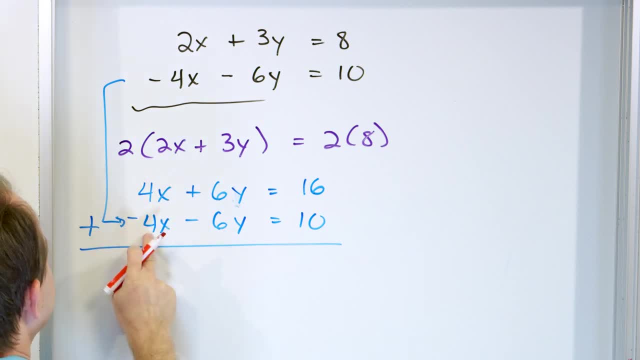 So when you have 4x plus a negative 4x, you get actually 0xs And 6 plus a negative 6, you'll get also 0ys, And when you add these together, you will get 10 plus 16, 26.. 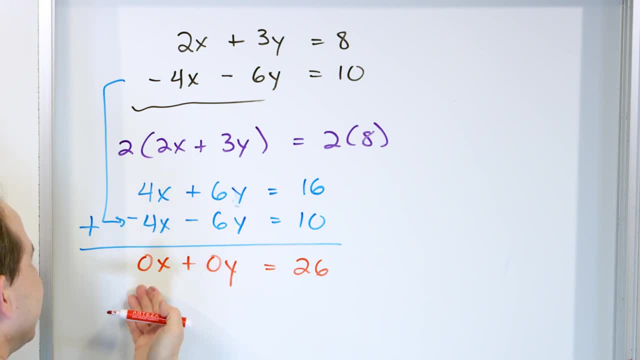 So what you have here is 0x And what you have here is 16.. 0x plus 0y, But this is really nothing. This is 0 is equal to 26.. Now, can it ever be true that 0, the number is equal to 26?? 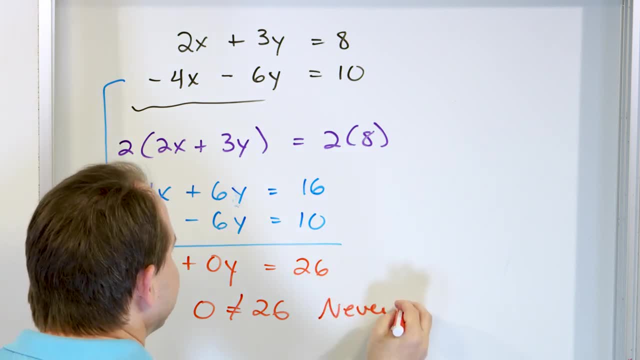 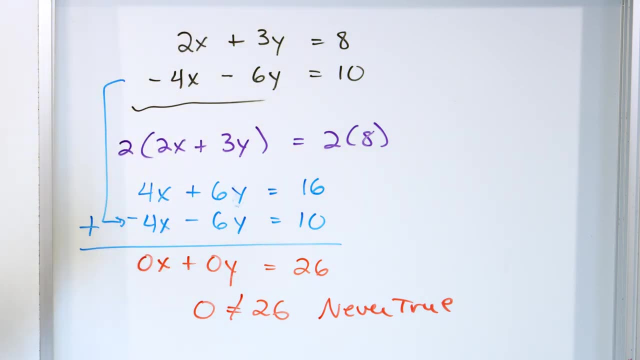 No, It's never true, Never true. So in the course of doing all of these legal things, we know we can multiply this by 2. We know we can add them together, But when we do it we get a nonsense answer. 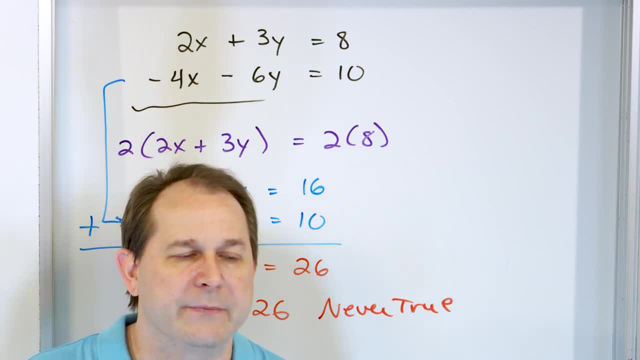 You see, sometimes you read in the history of science. people say, well, they predicted this or that particle, or they predicted this law of answers, Or they predicted this law of antimatter or whatever. Or you might say this is impossible. 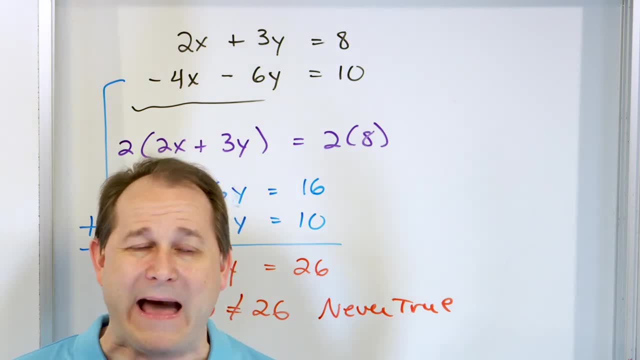 The law predicts this won't happen. This is the kind of way in which math can predict things. You see, the answer that you get is nonsense. It cannot be true. So these equations are weird in some weird way that makes them not true. 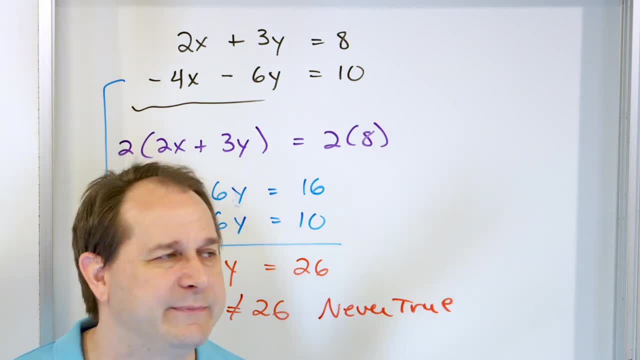 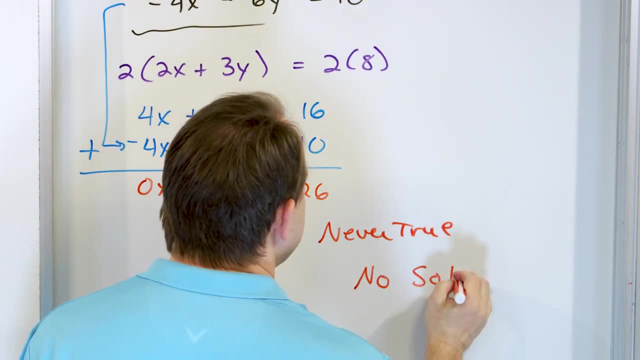 What it means is there is no point where they are both true at the same time, Because when you add them together, you get something that's nonsense. So what you get is no solution, And what this means is these are parallel lines. I'll put a little parallel there. 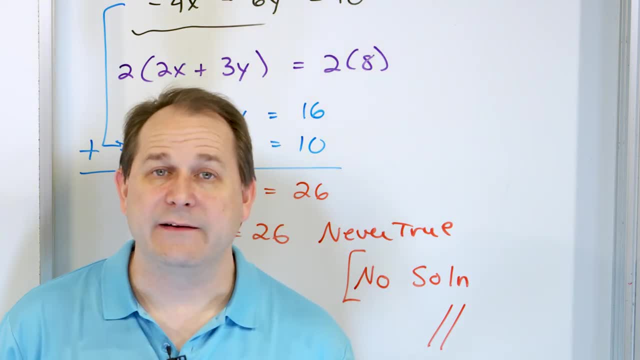 So if you were to graph the first line and you were to graph the second line, you would figure out that they have the same slope. I encourage you to do that. Go ahead and plot both of those and you will find out that both of these lines are actually parallel. 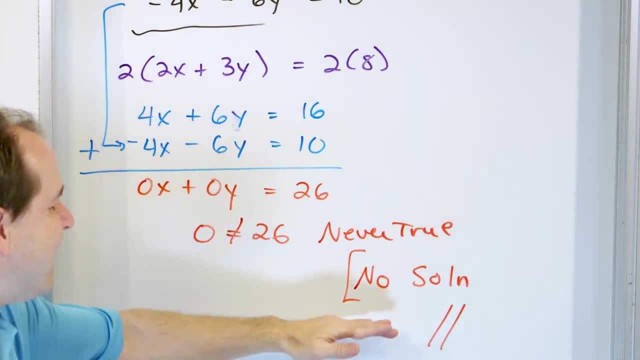 Put them into mx plus b form and they'll be parallel, And that is why they have no solution, And the way this falls out in this solution technique is that you'll get an answer. that, basically, can never be true, And that's what I wanted to point out for our last problem. 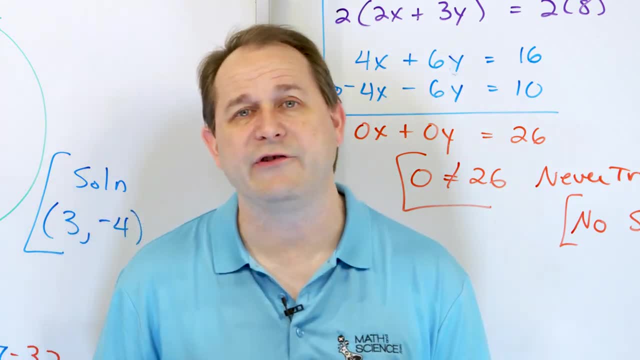 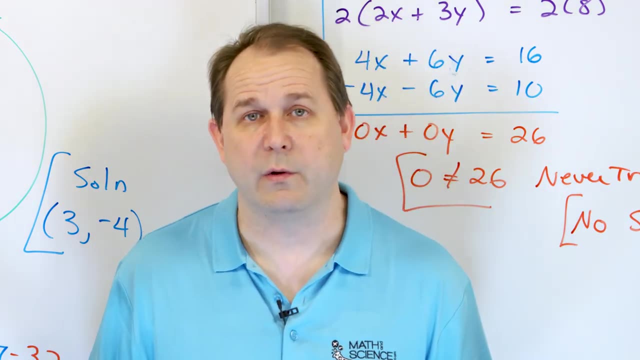 So in this lesson, we've learned how to solve systems of equations by elimination, by addition, And we've conquered the cases of when we have a solution, when we don't have a solution, and so on. What I'd like you to do now is practice all of these.